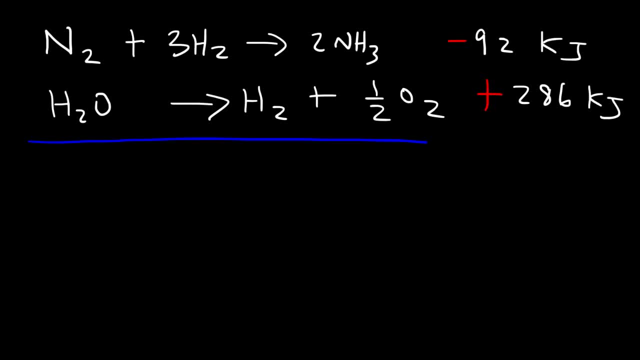 reactions. how can we calculate the enthalpy change of this reaction? Ammonia and reacting with oxygen gas, producing nitrogen gas and water. so Hess's law states that we can use these reactions, adjust them in such a way to get the enthalpy change of this reaction. but how do we go about doing it? so here's what. 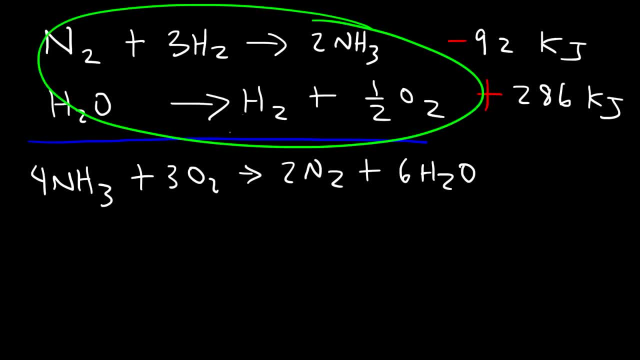 we need to do? we need to adjust these two reactions in such a way that when we add them, we get this reaction, and then we need to adjust these values accordingly, and when we add those numbers, we're going to get the enthalpy change for this reaction. and that's how we're going to do it. so it needs to. 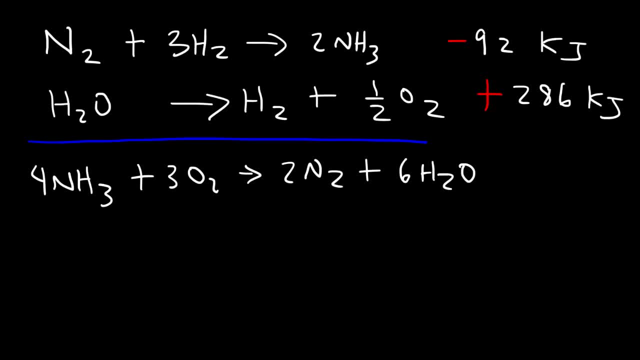 focus on the right stuff. so in reaction one and two you want to focus on the reactions and products that appear only once in those two reactions. for example, nitrogen gas is only found in equation one, not an equation two, so you want to focus on n2 hydrogen gas. it's 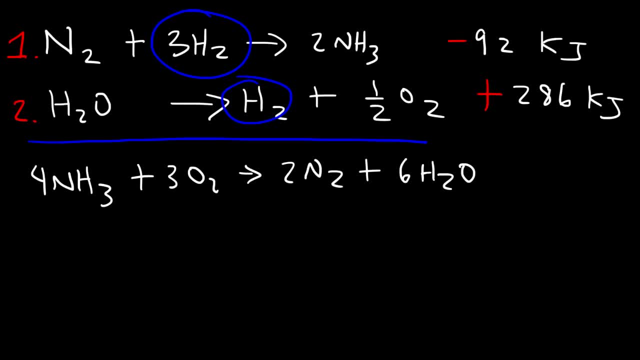 found in both of these two equations. so you do not want to focus on h2. if you do, it's going to make your life a lot harder. so notice that nitrogen gas is on the left side, but we want it to be on the right side and we need a coefficient of two in front of it. 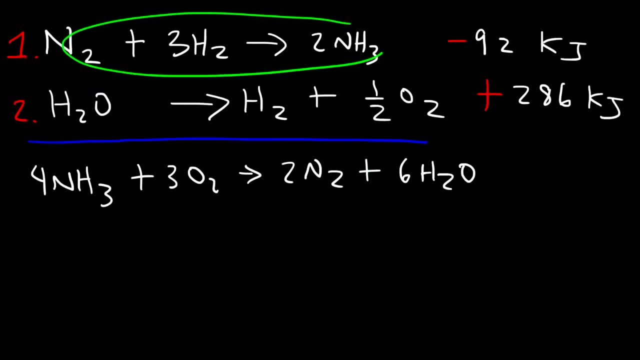 so what I'm going to do is I'm going to reverse this reaction and multiply it by two. whenever you reverse reaction, you got to change the sign, and if you multiply this reaction by two, you need to multiply the enthalpy change by two. so I'm going to 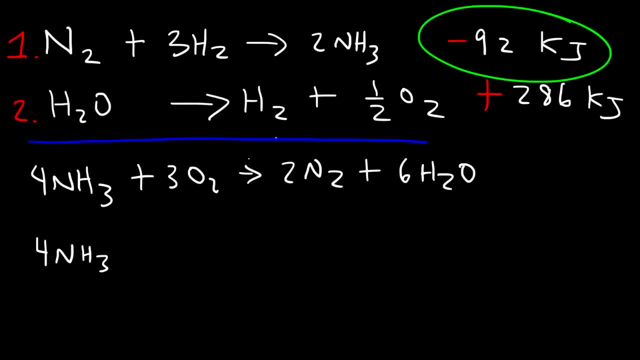 have four NH3. so this is now going to be on the other side, and if you multiply two NH3 by two, you should get four NH3 and this is going to yield two NH3 plus three times two is six, so that's going to be six H2 and the enthalpy change is 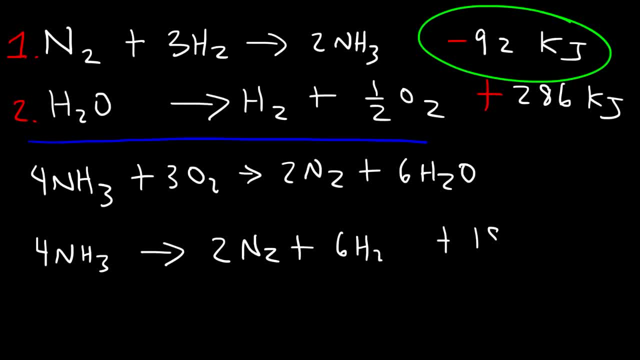 going to be positive. 184 kilojoules, that's 92 times two. now let's focus on this equation. should we focus on water, H2 or oxygen? you can focus on water or oxygen, but you don't want to focus on H2 because it's found in these two equations. 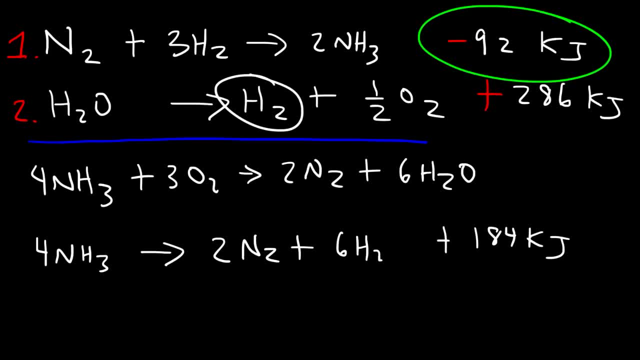 so I'm going to focus on H2O. notice that in the net reaction we have six water molecules on the right side. here we only have one on the left. so we need to reverse it and multiply by six. so six times that is going to be six H2 and then 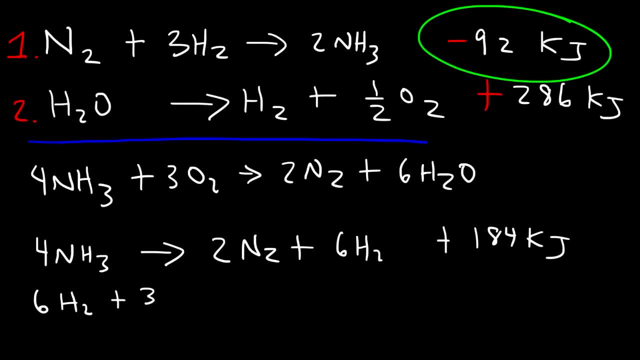 six times a half O2, that's going to be 302 and that's going to produce six water molecules. so we're going to change: the sign is going to be negative 286, and then we're going to multiply it by six, so that's going to be negative 1716 kilojoules. so 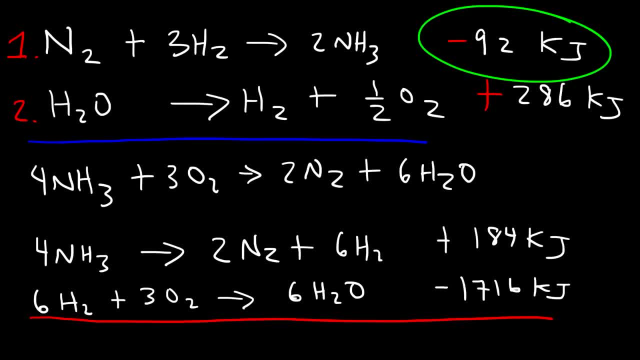 now let's add the two reactions and we need to make sure that we get the net reaction. so we have four NH3 on the left, that's to the left of this arrow. so let's rewrite it here: four NH3 and notice that the six H2 molecules they cancel because they're the same on. 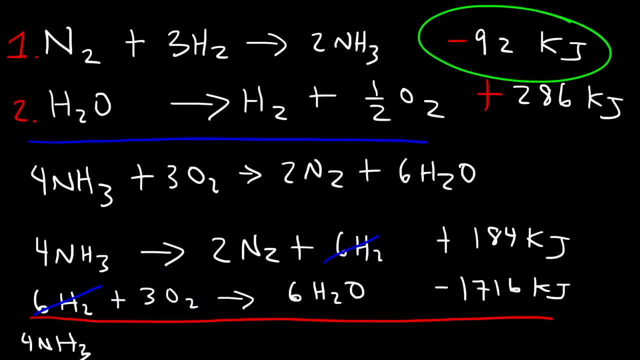 both sides. on the left we have 302- that's left of that arrow- and then on the right side we have two N2 and six H2O, which is the same as what we have here now, since we add equation one and two to get this reaction. 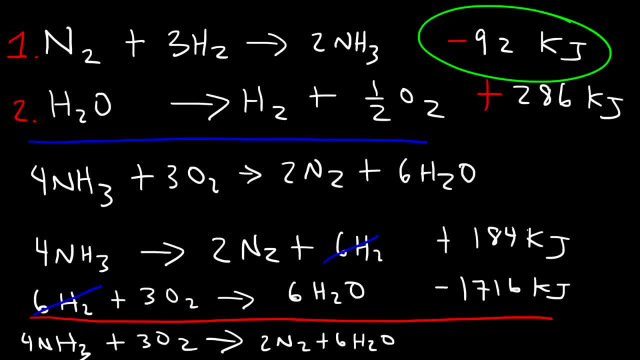 to calculate the enthalpy change of that reaction according to Hess's law, we just need to add these values, so it's 184 plus negative 1716, so the answer is going to be negative 1532 kilojoules, and so that's how you can use Hess's law. 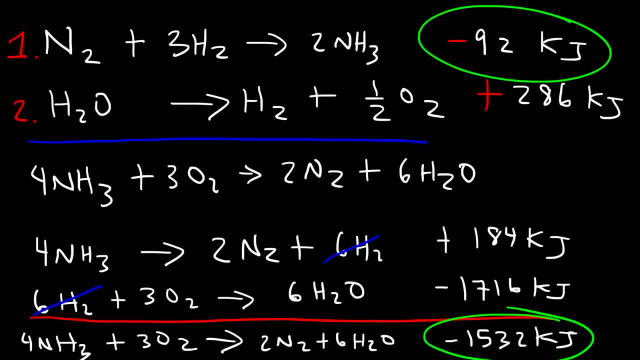 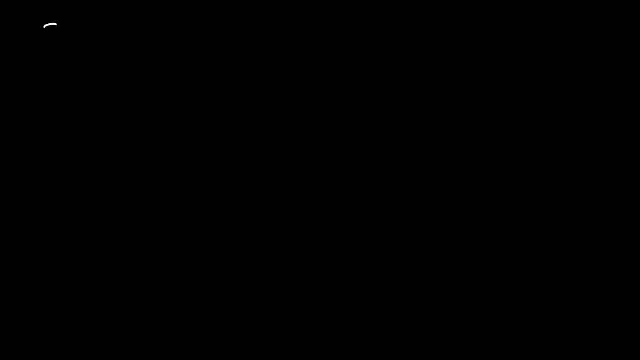 to calculate the enthalpy change of a reaction if you know the enthalpy changes of other reactions? here's another example. let's say that water decomposes into hydrogen gas and oxygen gas. let's say that that process requires positive 576 kilojoules of energy and 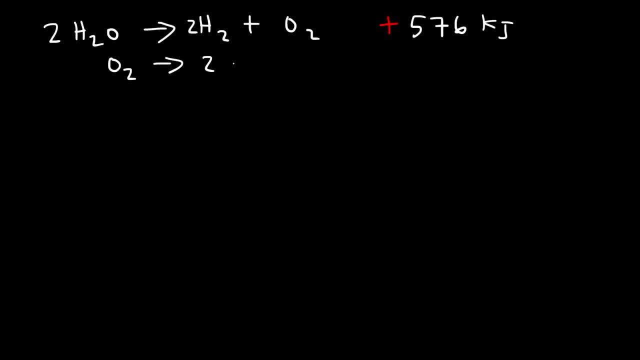 then oxygen breaks down into atomic oxygen with an input of positive 495 kilojoules. so with this information, use Hess's law to determine the enthalpy change of this reaction: hydrogen gas plus atomic oxygen produced in liquid water. so feel free to pause the video as you try that example. 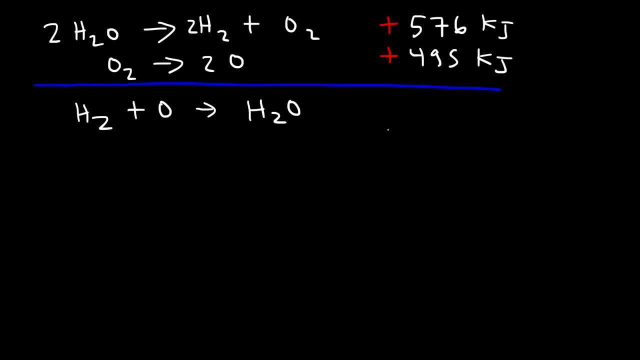 so what's the first thing that we need to do? in this example, it's best to identify which species to focus on. I'm going to focus on hydrogen gas. notice that we have two of it on the right side, but we need one of it on the left, so we 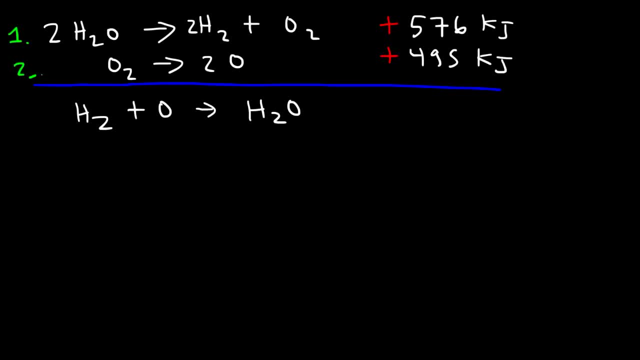 gotta multiply the first reaction by a half and we need to reverse it. so once we reverse it it's going to be H2 and you gotta divided by two, so H2 plus one half O2, producing one water molecule. now I need to make one small correction. 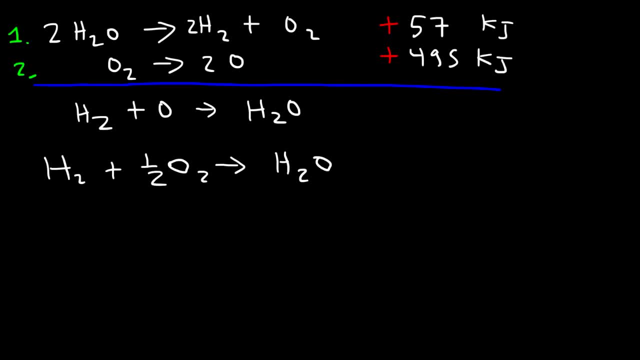 that should be a two, not a six. now we need to change the sign and we have to divide that number by 2. 572 divided by 2 is 286, so this is going to be negative 286 kilojoules. now notice that we have. 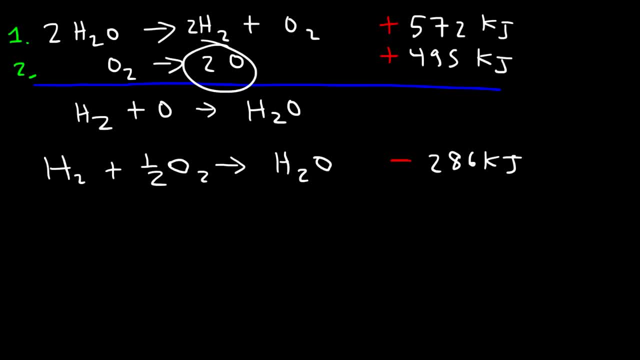 one oxygen atom on the left side and here we have two on the right side. so we need to reverse that reaction. and divided by 2 as well, so it's going to be Oh turning into one half, oh two. so it's gonna be negative 495 divided by 2, which. 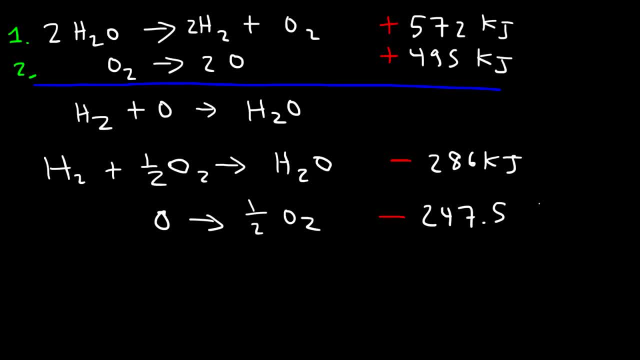 is two hundred and forty seven point five kilojoules. so now let's add the two reactions, so these two numbers will, those two things will cancel, so it's gonna be h2 plus Oh. turns into a liquid water, so negative two eighty six plus negative two forty seven point five is negative five. 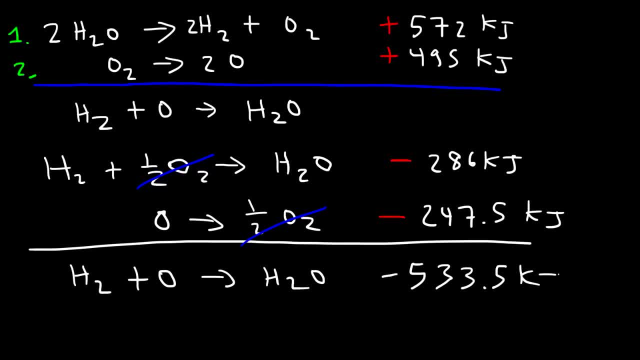 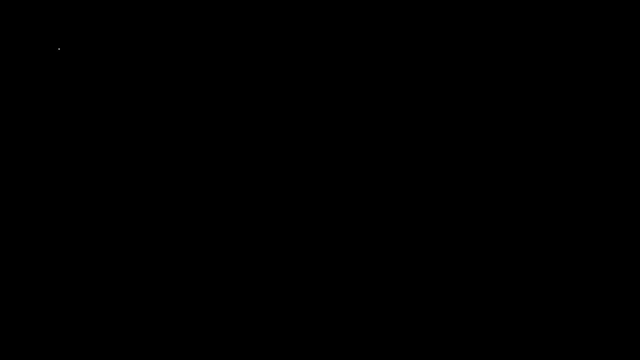 hundred thirty three point five kilojoules, and so this is the answer. now let's consider one more example. so we're going to have two ozone molecules decomposing into three oxygen gas molecules, and the energy for that is going to be negative 427 kilojoules. I'm gonna have to write small, cuz there's gonna be more. 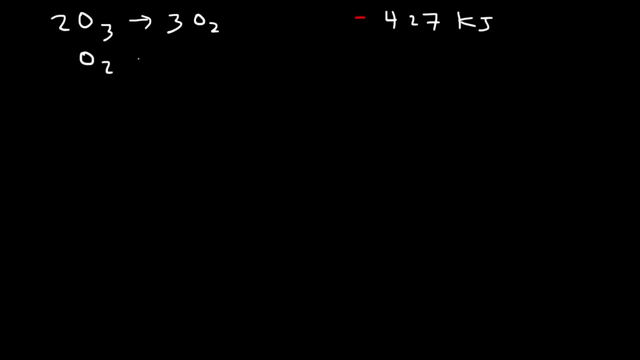 reactions in this one and then the last one. now, in the next one, oxygen gas decomposes into atomic oxygen, and so the energy change for that is positive 495 kilojoules. and then finally, we have nitrogen monoxide reacting with ozone to produce nitrogen dioxide plus oxygen gas. 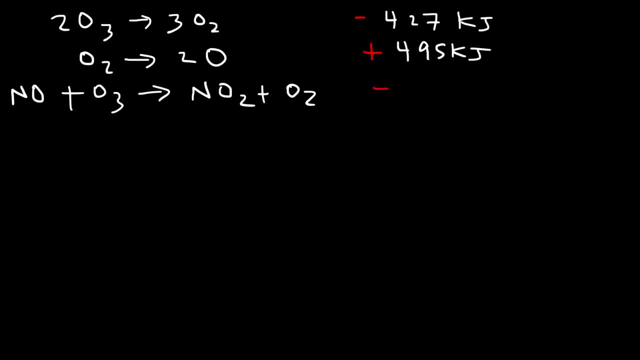 and so this is going to be negative one hundred and ninety nine kilojoules. so, with this information, go ahead and determine the enthalpy change of this reaction: nitrogen monoxide plus atomic oxygen turning into nitrogen dioxide. so go ahead and try it. so let's call this: 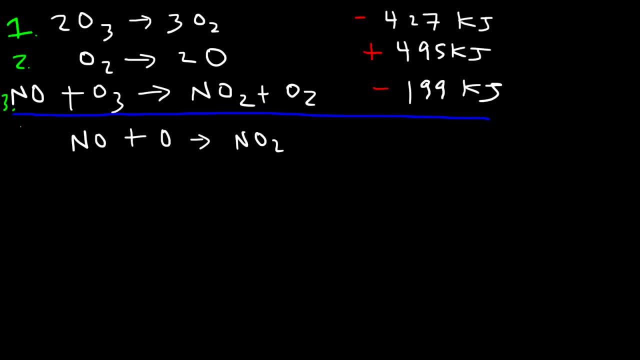 equation one, two and three. so what should we focus on? I'm gonna focus on equation three, so notice that I have nitrogen monoxide on the appropriate side. I don't have to change, so I'm going to rewrite equation three, and so the energy change is going to remain negative: 199 kilojoules now notice. 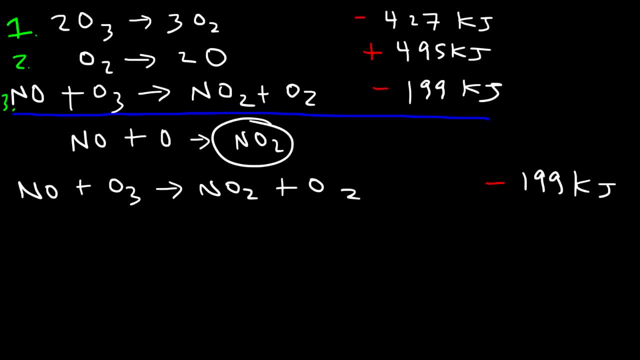 that nl2 is already in the appropriate side. so the next thing I need to focus on is atomic oxygen, which is only found in equation two. so I need it to be on the left side. so I have to reverse this reaction and multiply by half. so this is: 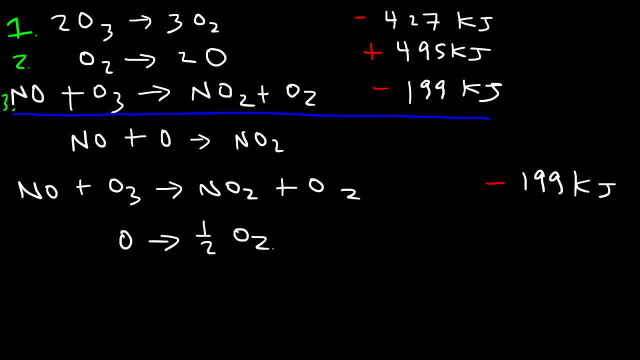 going to be 0, turning into 1 half O2, and so this is going to be negative. 495 divided by 2. we said it was 247.5. now notice that ozone and O2. they're found in other reactions. O2 is found in equations 2 & 3 and ozone is only found. 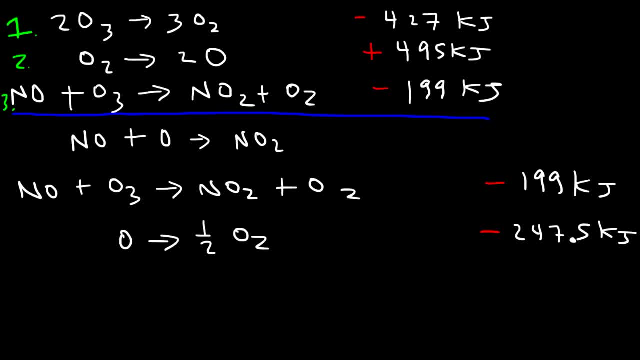 in one three. so I'm gonna focus on ozone now, because ozone is not in the norte action. that means I need it to cancel completely. so in this reaction, have one ozone molecule on the left side. if I want that to cancel, I need to have one. 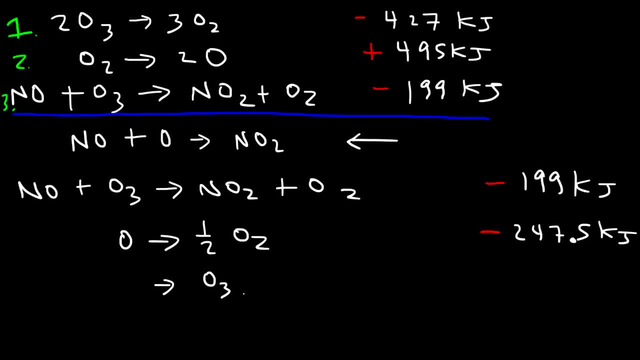 ozone molecule on the right side. so I've already used equation tree, going to focus on equation 1: Ka gear minuses equation 3, and this one is 2. so in order to get one ozone molecule on the right I need to reverse that reaction and multiply by half. so on the left I'm. 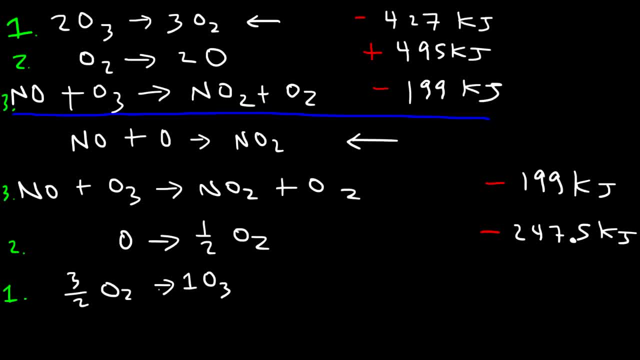 going to have 3 over 2 O 2, and it's going to change from negative to positive. and then I need to divide 427 by 2, which is two hundred thirteen point five kilojoules. so now let's add the reactions, so ozone will cancel. 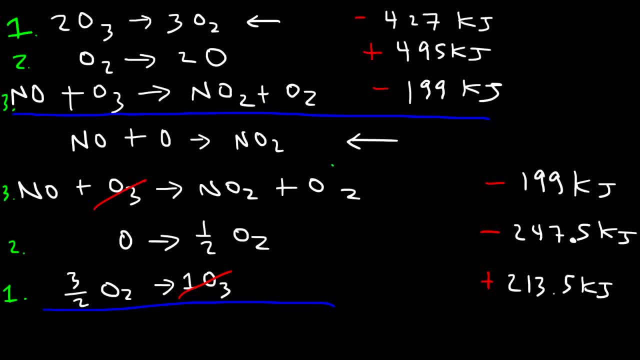 now, on the right side we have one oxygen gas molecule plus a half, so that's 1.5. on the left side we have 3 over 2, which is 1.5. so therefore this cancels with these two on the right. so what we have left over is NO plus O turns into NO2. so